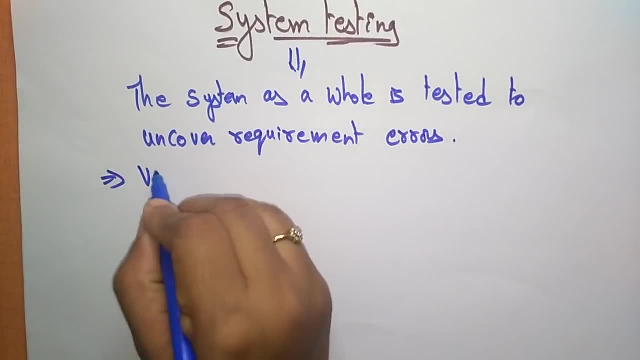 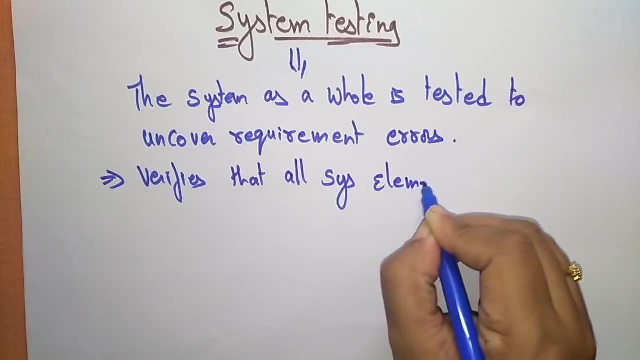 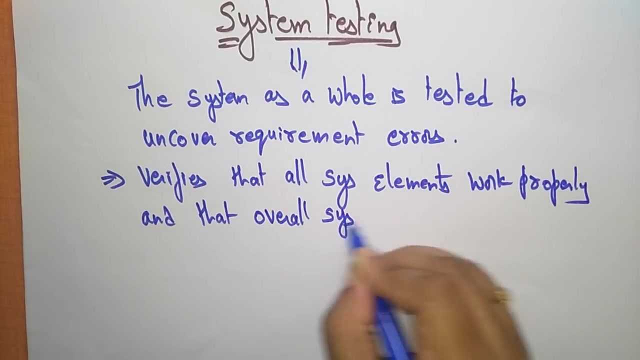 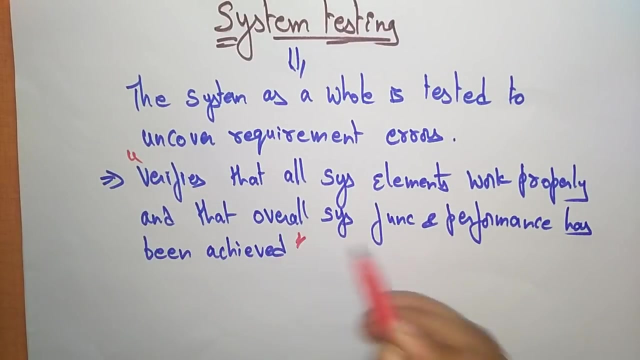 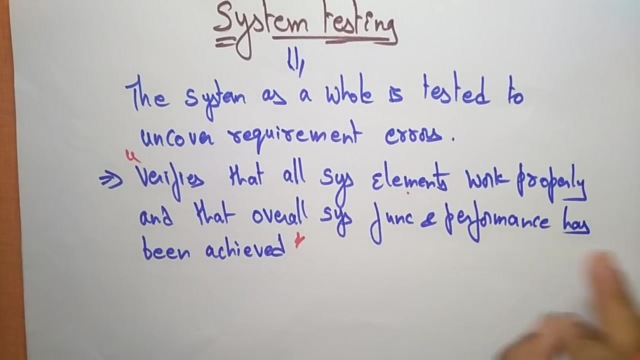 So this is the system testing, And this system testing verifies that all system elements work properly. It is going to check whether all the system elements work properly and that overall system function and performance has been achieved or not. So this is a main use of this system testing. The system testing is going to verify all the system elements work properly or not, And also it concentrates on overall system functions, performance and that has been achieved or not. Now let us see the different types of system testing. 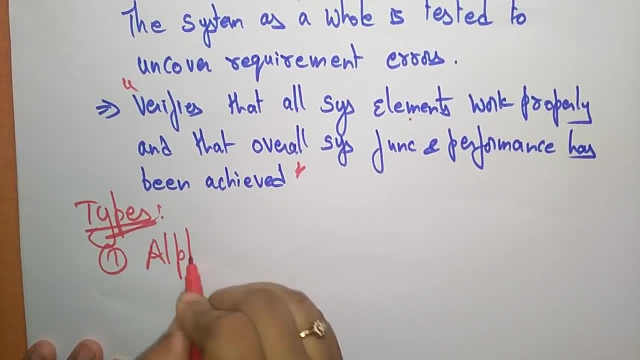 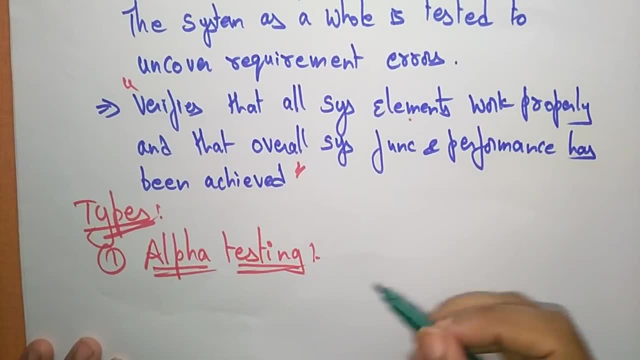 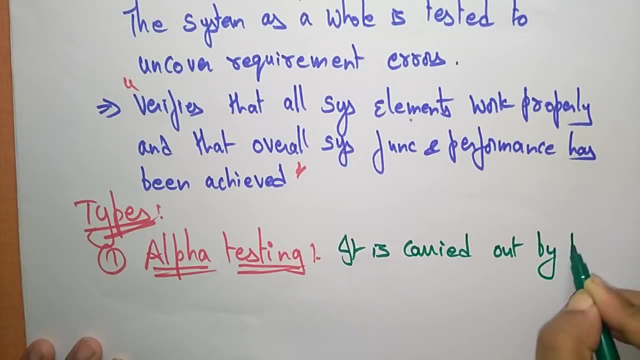 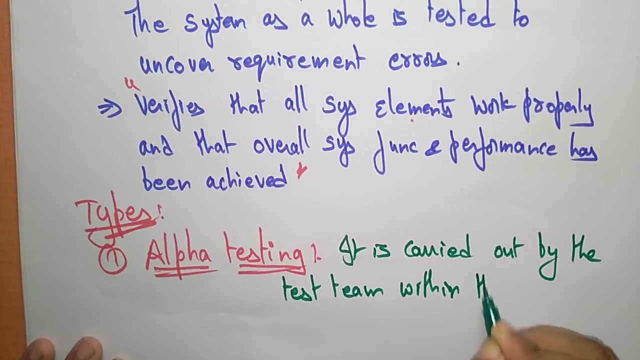 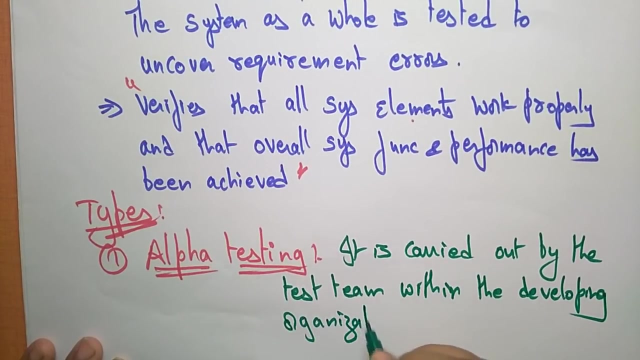 Different types. The first one is all for testing. So what is all for testing? All for testing. it is carried out. It is carried out by the test team Within the Developing organization. that is all for testing. Actually, we are doing the test on the whole system. So that I already said. 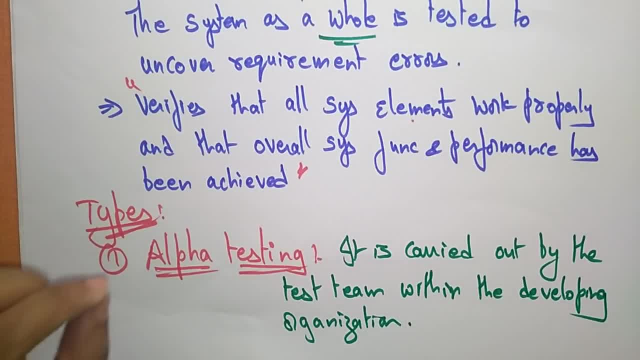 So here, what is the one type of System? testing is all for testing. that what it means. all for testing means the test is carried out by the test team within the development organization. So within the development organization, one test team was there. Those team are going to test. the system means the whole system is testing, only the test team. that too, within the organization, developing organization. So that is all for testing. 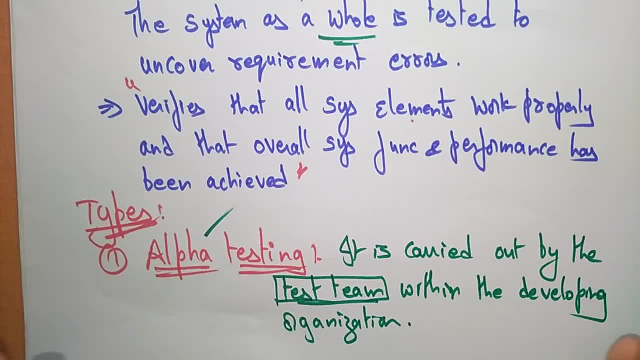 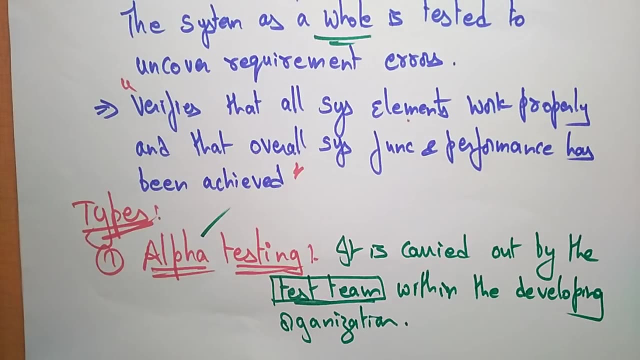 So whenever you are Asking about what is all for testing, a testing will be done within an organization by A specific test. a unseen that is all for testing means it is not tested by the other people outside people, only in the internal organization, The developing organization company. 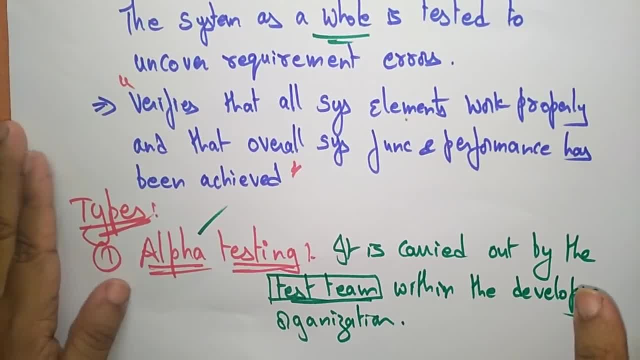 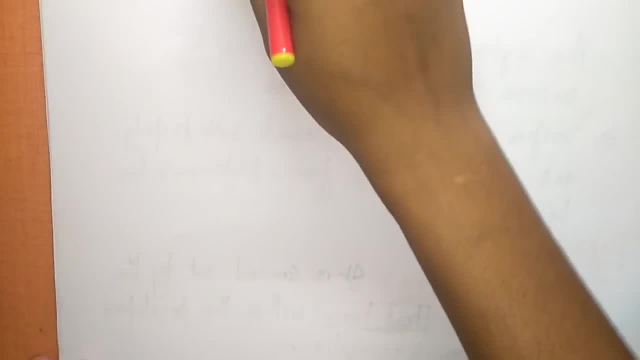 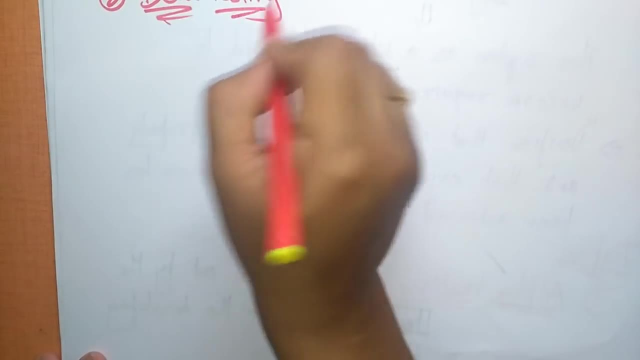 They just have a test team. Those people are going to test the system. that is Now coming to the next to these two. next, SL type of testing, that is, intercept. The second is beta testing. So where this beta testing will be done, The whole system has. 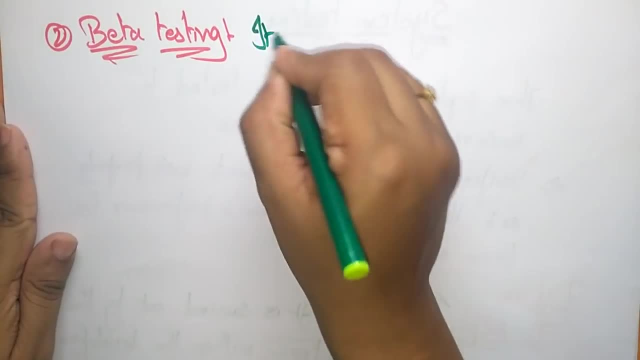 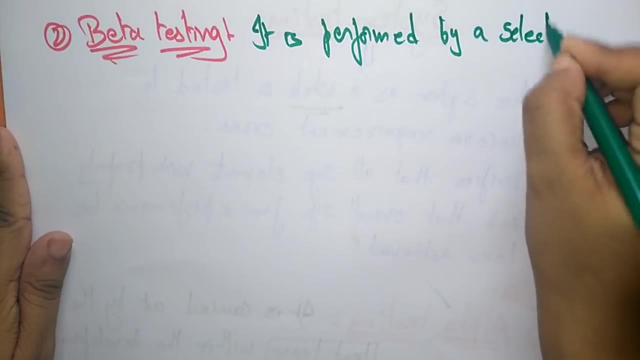 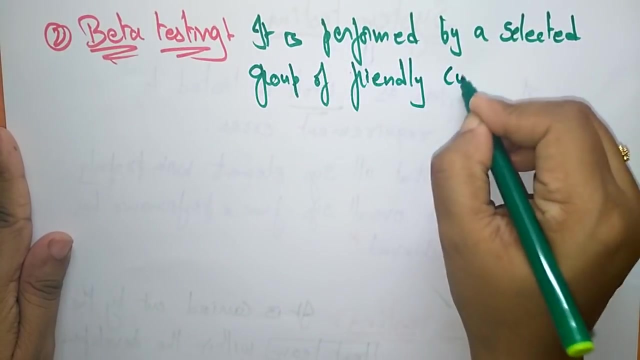 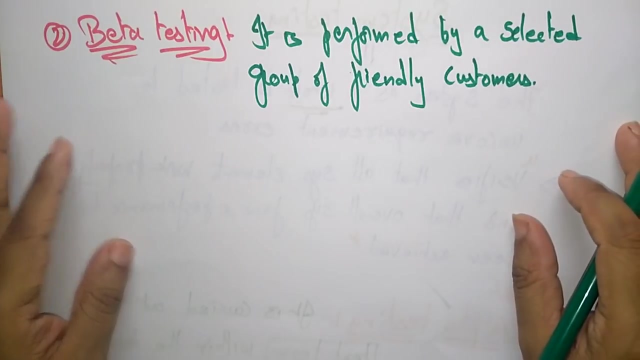 to be tested, Beta testing. it is performed by. it is performed by a selected group, selected group of friendly customer. So, instead of the organization people or instead of the testers in any developing organization, this beta testing is nothing, but it is performed by the complete 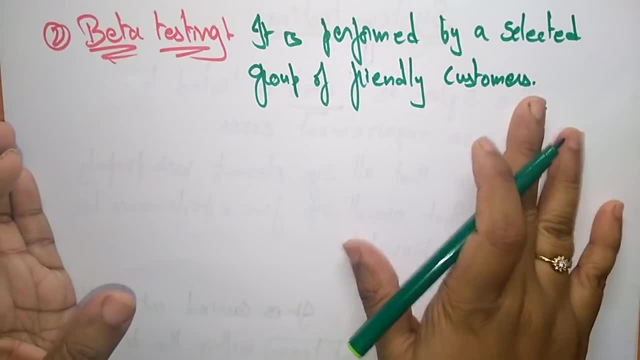 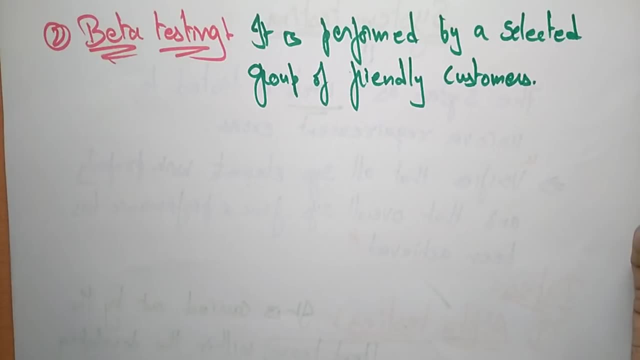 system is going to perform by selected group of friendly customers. means other people, other customers who are friends to you. okay, So you are trusted on them. okay, Whenever you trust on them, you are just asking the asking them: please test my product. is it properly working or not? Means you are just giving. 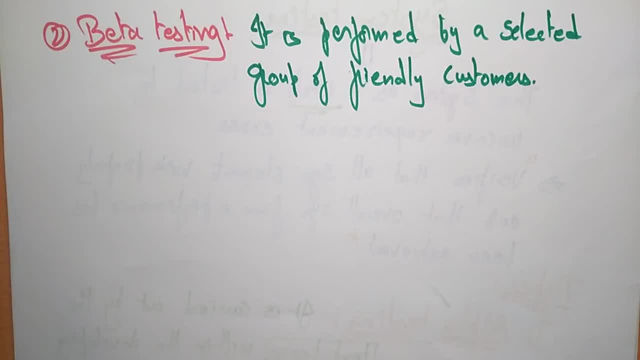 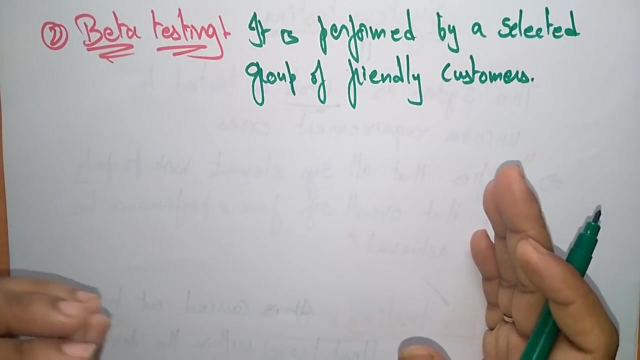 different ideas, different views of different people means whenever you check your system, you would see that it is everything is okay. But if another people, different, other people which are not involved in that product, if they are operating, they will see what the problem in. 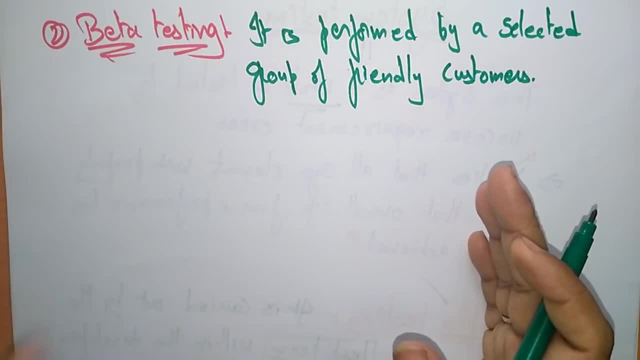 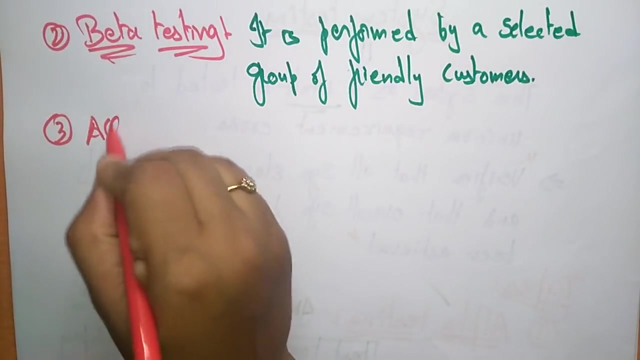 that. So that's why, in the system testing, while if you want to deploy the product, if you want to deliver your complete product, you are going to test in different ways. That is alpha testing, beta testing and next one is acceptance testing. So this 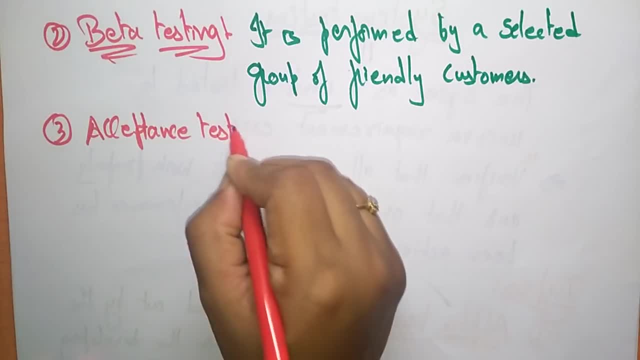 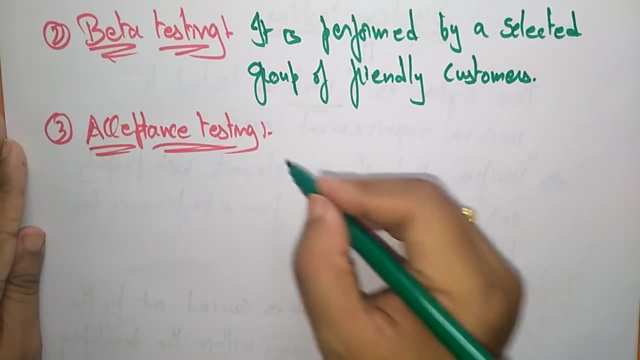 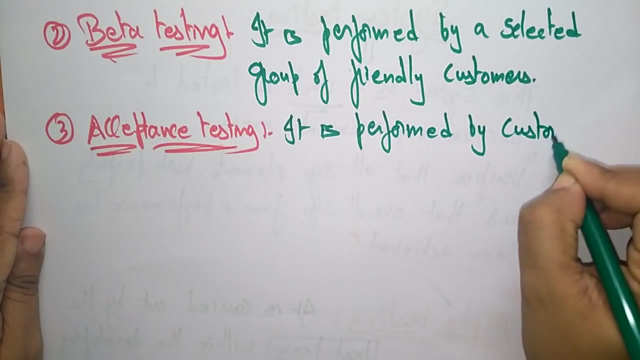 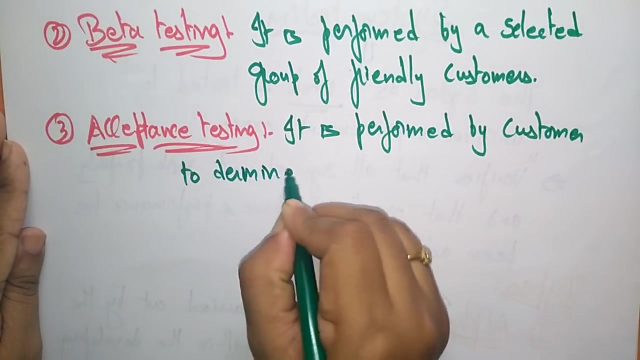 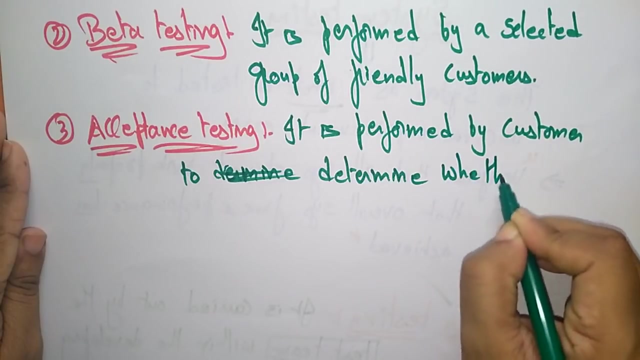 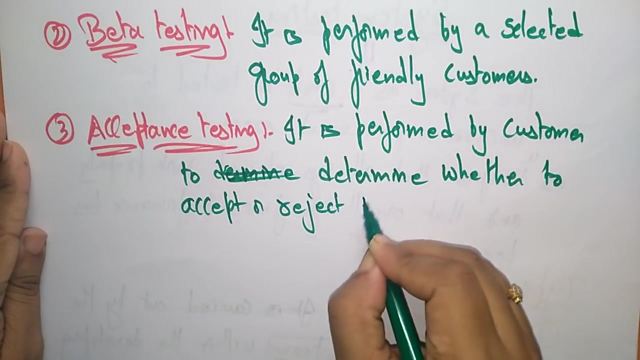 acceptance testing is nothing, but it is the only the customer who is going to take the product. that person is going to test. It is per Toy who is going to test. It is performed by customer To determine, to determine- sorry, to determine- whether to accept or reject, to accept or reject the delivery of system. 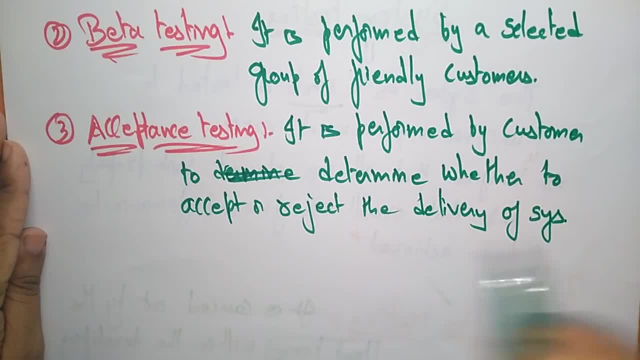 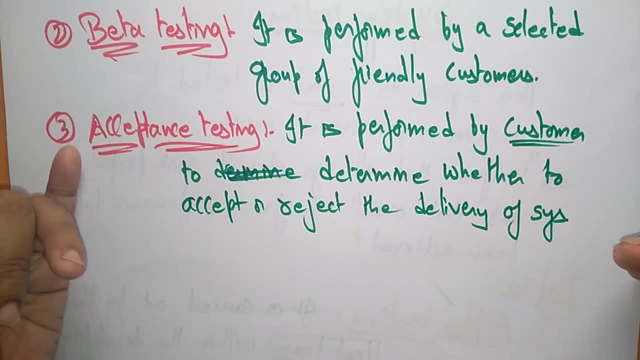 So this is a test done by the going to, done by the customer itself. If in the system testing, another type of testing is the accept and testing. So this all testing has to be executed. So whenever all the testing cases are satisfied, then the product is a very good working stage in a good working stage.